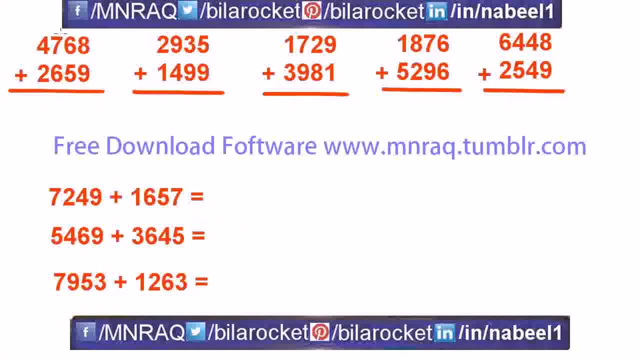 So right here we have the ones place, we have the tens place, the hundreds, and the thousands. It's important to keep the ones in the ones place when they're stacked on top of each other. 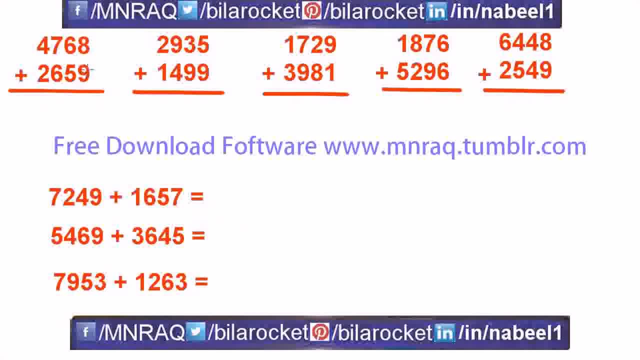 So we're adding big numbers like this. We start in the ones place. You add 8 plus 9. So 9 and 8 equals 17. You carry over the 1, bring down the 7. 5 and 6 is 11 plus 1 is 12. Carry over the 1, bring down the 2. 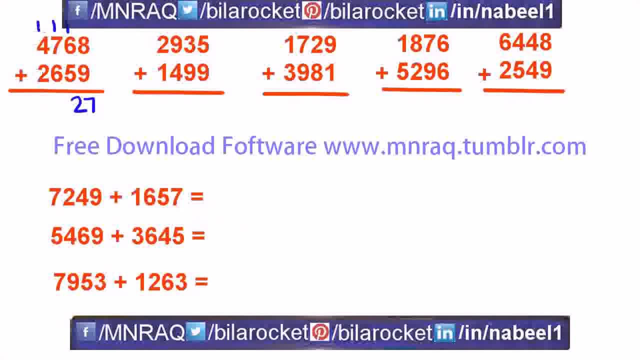 7 and 6 is 13 plus 1 is 14. 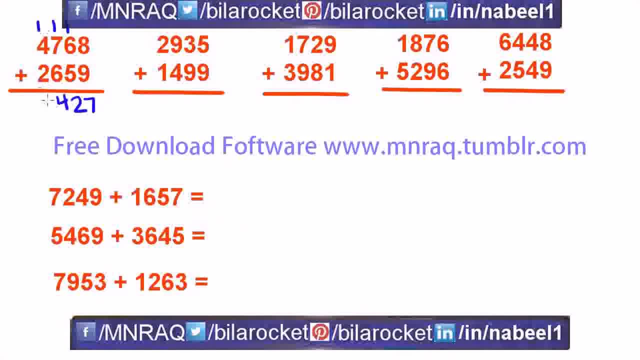 And 4 plus 2 is 6 plus 1 is 7. 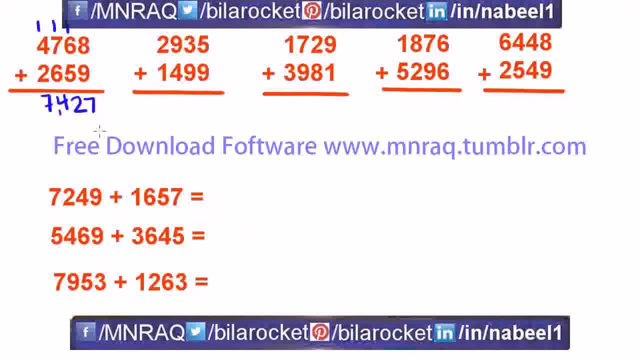 So there's your product, 7,427. Same deal over here. We start in the ones place. 5 and 9 is 14. Carry over the 1, bring down the 4. 9 and 1 is 10 plus 3 is 13. 9 and 1 is 10 plus 4 is 14. Carry over the 1, bring down the 4. 2 and 2 is 4. So you got 4,434. Alright, 9 and 1 is 10. 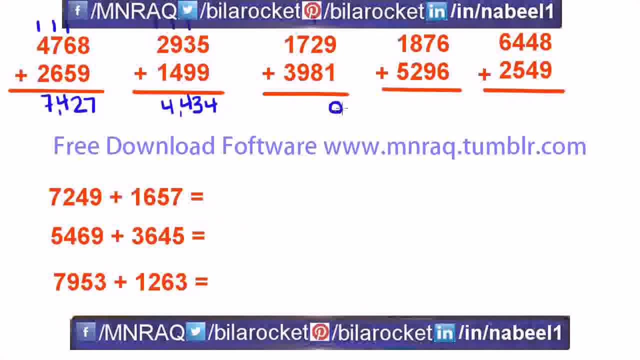 Carry over the 1, bring down the 0 as a placeholder. 2 and 8 is 10 plus 1 is 11. 9 and 1 is 10 plus 7 is 17. Carry over the 1, bring down the 7. You want to make sure that you keep it right underneath. So 3 and 1 is 4 plus 1 is 5. 5,710. Over here we got 6 and 6 is 12. Carry the 1 again, bring down the 2. 9 and 1 is 10 plus 7 is 17. Carry the 1, bring down the 7. 8, 9, 10 plus 1 is 11. 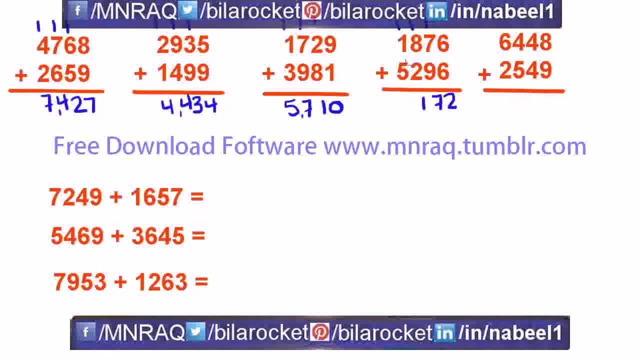 5, 6, 7 and 7 is your last number. So it's 7,172. 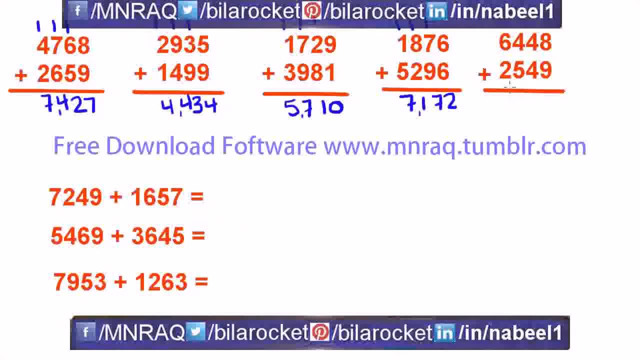 Over here we have 9 and 8. Which is 17. Carry over the 1, bring down the 7. 4 and 4 is 8 plus 1 is 9. You just bring down the 9 since it's a single digit number. 4 and 5 is 9. Bring down the 9 again. No need to carry over a number.